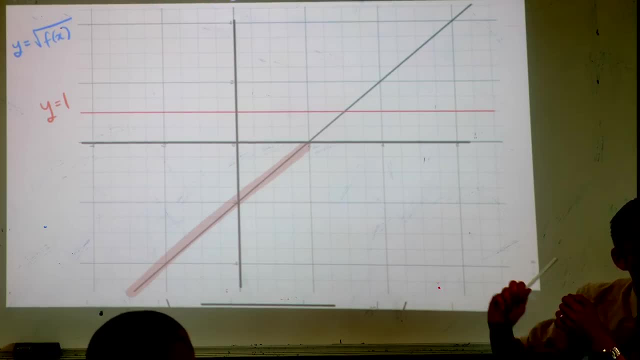 What's the square root of 1? It's 1.. So anywhere that our original function intersects with y equals 1, like say: right there, when you take the square root of that, you're also going to get 1.. 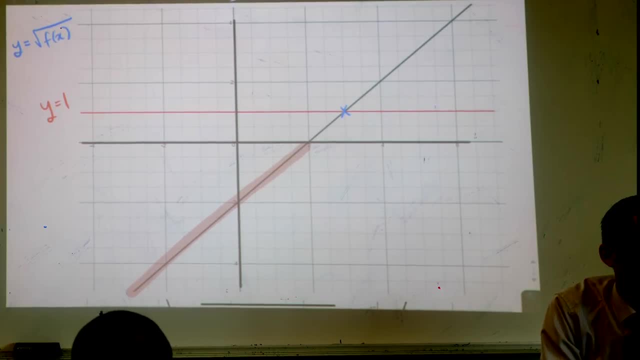 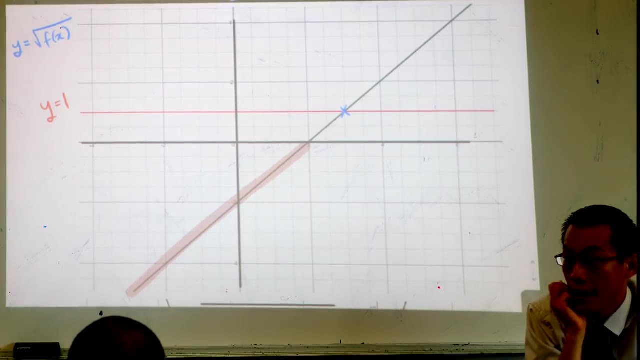 The square root of 1 is 1.. Think back to all of the graphs and transformations we did in the last few lessons. What other values for this function are important, not just 1? The x-intercept. The x-intercept is very important. 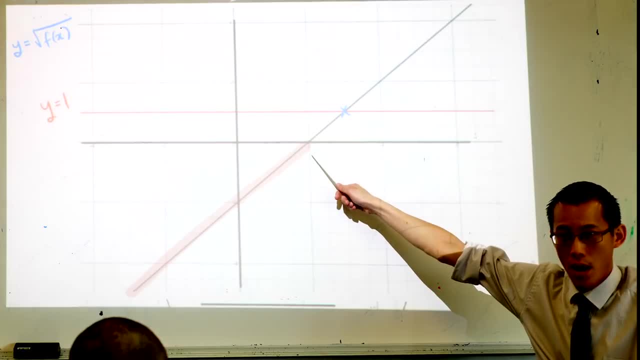 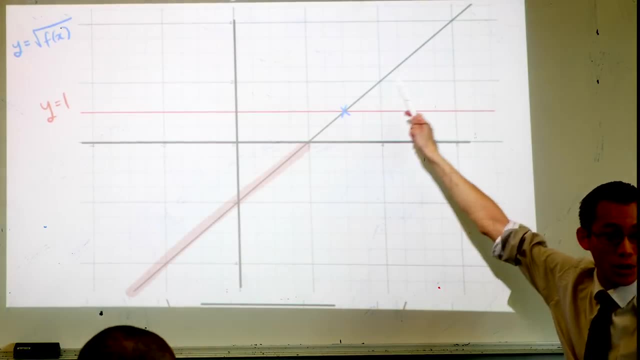 For y equals 0, which is just there, right? why is that significant? What's the square root of 0? 0.. 0.. Okay now, for reasons that will become clear in a second, see how I've got crosses here. I'm going to draw three more crosses over here. 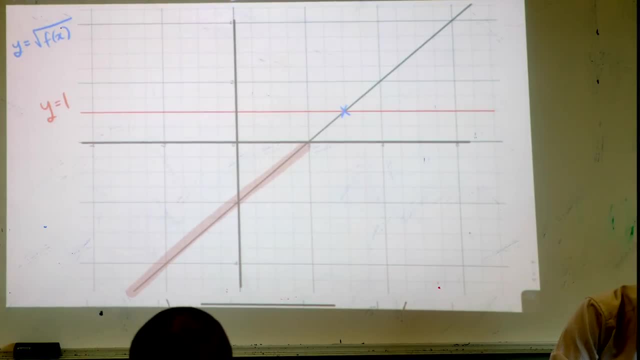 I'm going to ask you to draw this guy here. instead of a cross, draw a nice big fat dot. I'll explain in a little bit, Or maybe you can explain in a little bit, why I'm putting a fat dot there rather than just an x like I usually do. 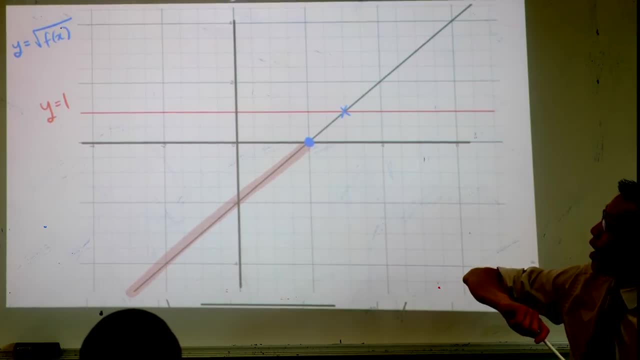 Okay, so I've got an x there. I'm looking now, for these are like all of the points that are usually important. I'm now looking for any values that are on the graph which I know I can take the square root of and get a nice number out, right. 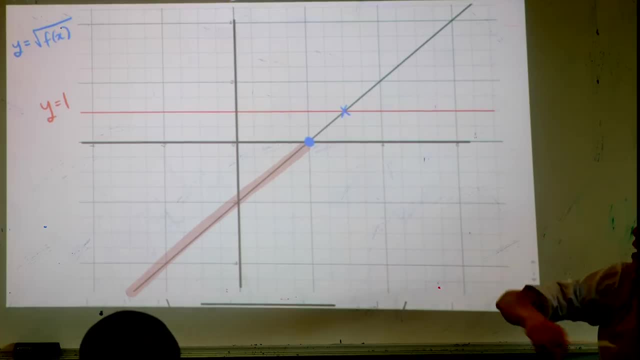 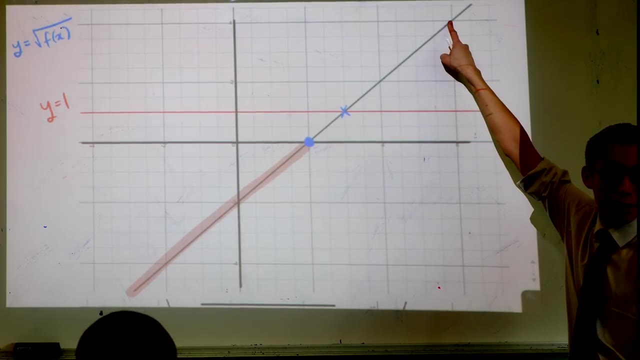 So you can see 4 right at the top there, right? Can you look what's the x value that corresponds to? y equals 4? It's 6.. It's 6,, very good. So over at x equals 6,, y is equal to 4.. 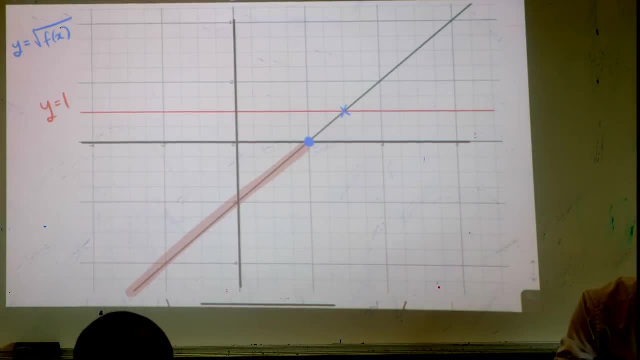 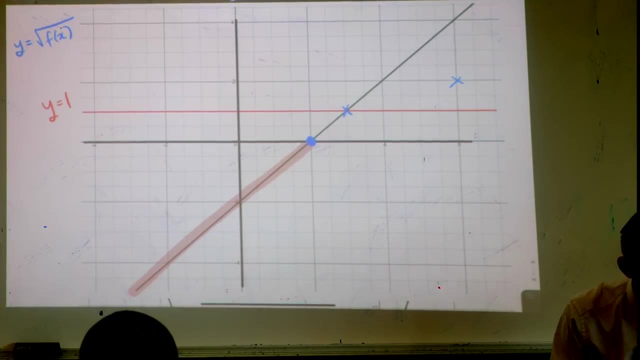 So when I take the square root of that, I will get 2, which should be right there. So go ahead and put an x there, Okay, If you want to. you kind of could go in between. So, for example, I happen to know that the square root of 2, there's 2 there- the square root of 2 is about 1.4.. 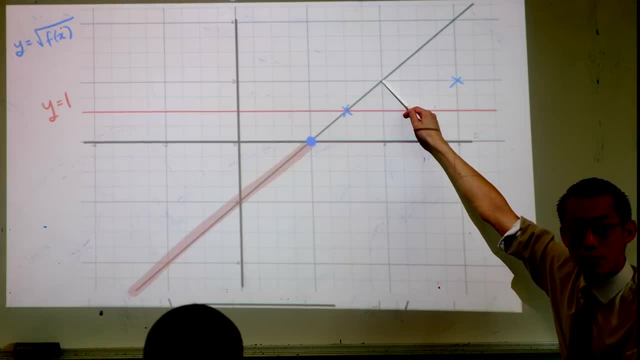 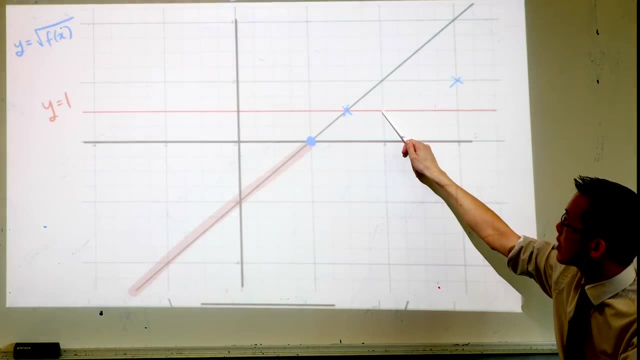 You can go chuck that into your calculator and get something out of that. So if that's 2, then when I take the square root of this y value, I should go down. I think 1.4 would be about that's 1, isn't it? 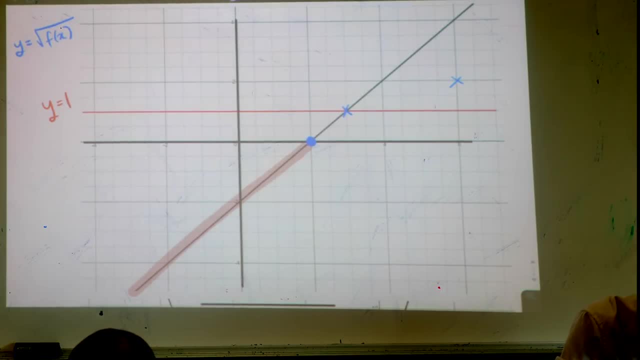 So 1.4 is about here, just below that extra line. So go ahead, Let's put another cross in. Okay, So you can kind of see there's a shape happening over here. We can join up these dots predictably. 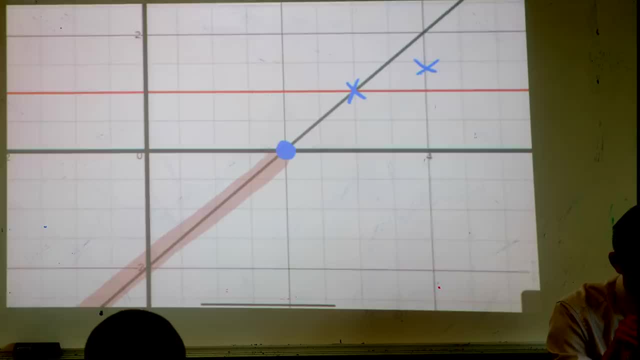 Before we do that, there's one more cross I want to put in And I'm going to cheat by zooming in, which I know you can't do, But do you remember I'm actually going to go back to, because I think I have it on this particular thing. 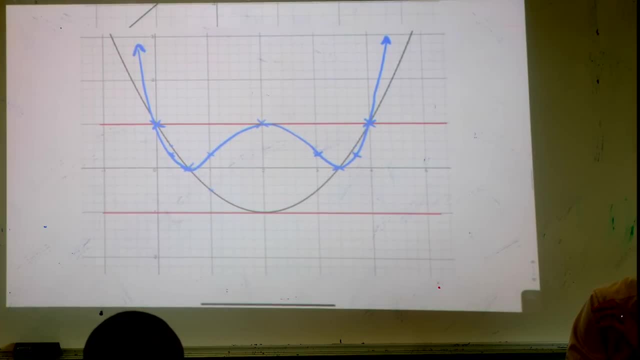 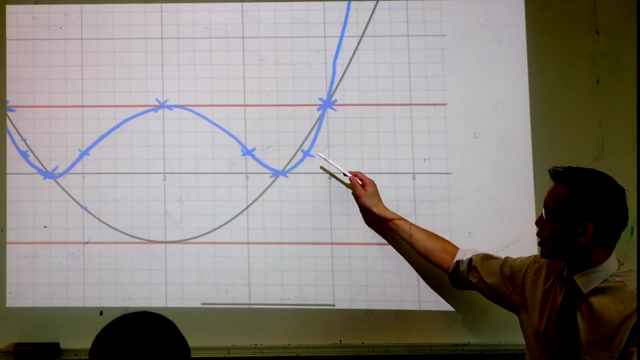 When we were squaring. will this one do? Yeah, this is a good one. Okay, So this is when we were squaring functions. Okay, So I want you to look and see if you can tell this again: is the y equals 1 line? 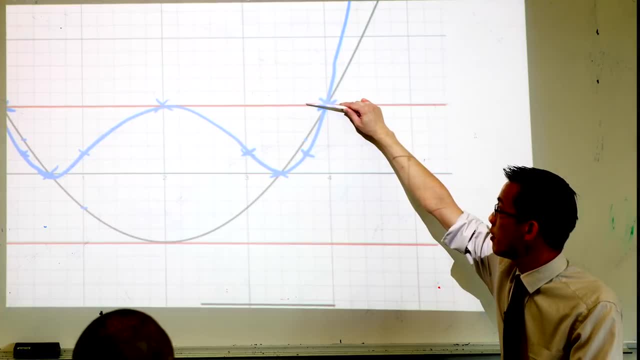 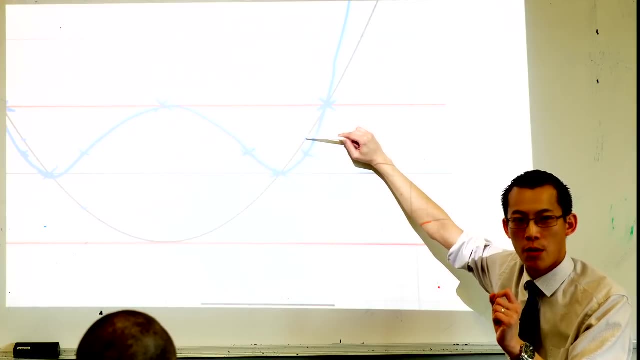 Okay, So what y value does this look like here? That's 1.. This is like. this is just a half right, It's halfway up to 1.. And then do you notice what point did I plot when I was squaring? 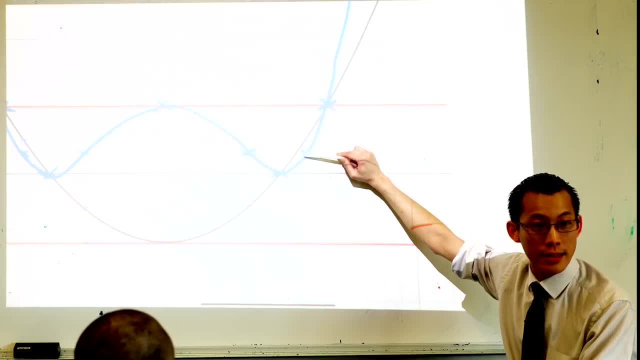 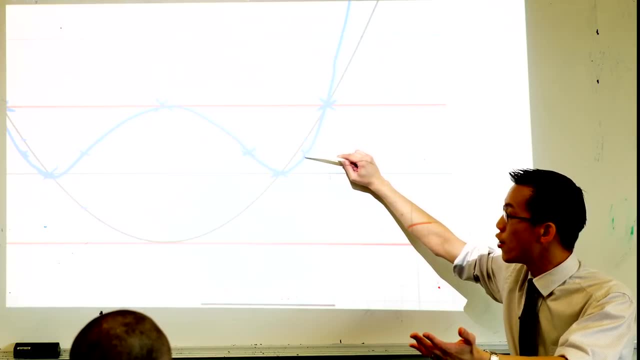 Because you do a half, you square it. what do you get? A quarter like that? right? When you're squaring, a half becomes a quarter, But right now I'm taking square roots, So I should go in the opposite direction, right? 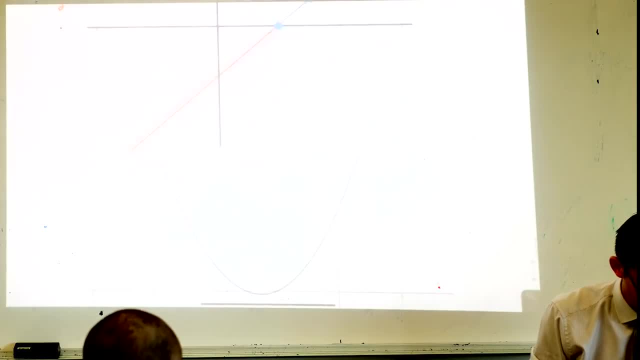 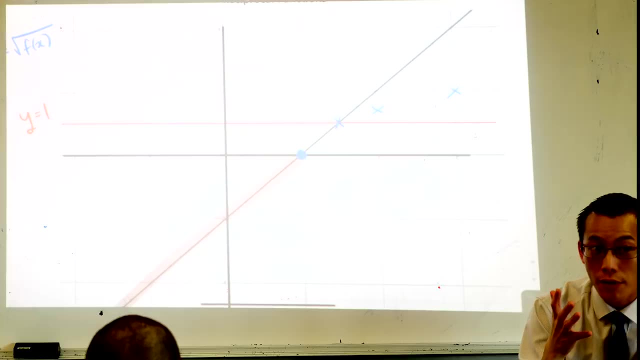 If I can find a quarter, Let's have a look at the graph we're looking at now. If I can find a quarter on here, the square root of a quarter is a half right. Where's a quarter on this? Can you look and find it? 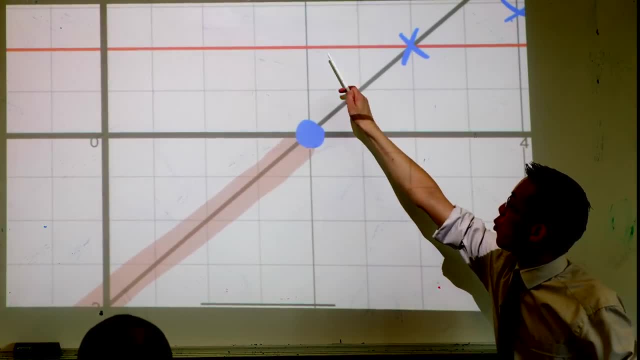 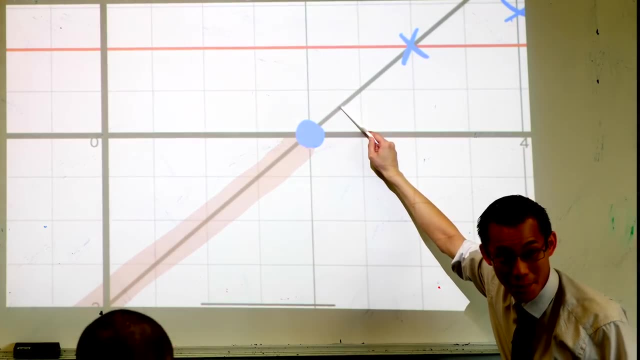 It's pretty close in right. So if this is 1, that makes this a half, That makes this yeah. so I think this is a quarter. Do you see that? I know you've got to like put your face right up to the page, but there he is. 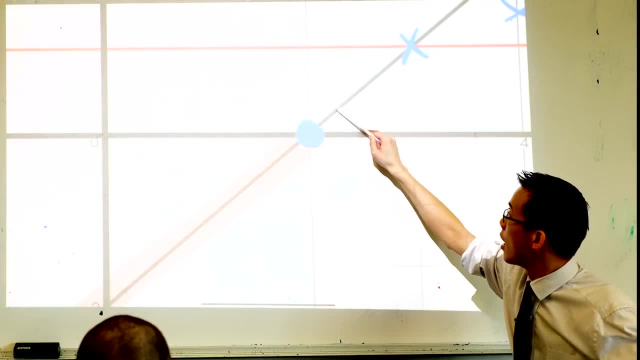 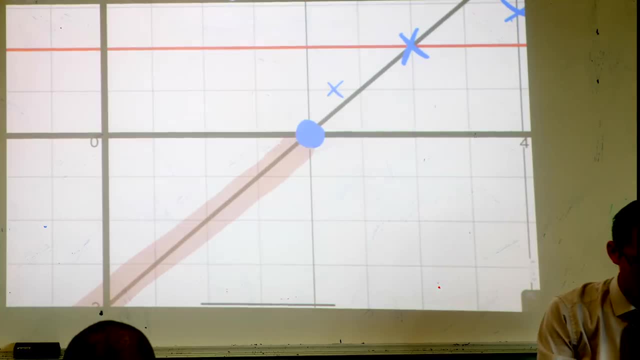 So there's a quarter. What's the square root of a quarter? It's a half, So I'm going to put an x just above there. Okay, Whoops, that's highlighting, sorry, There you go. Okay, now I think we can join this together. 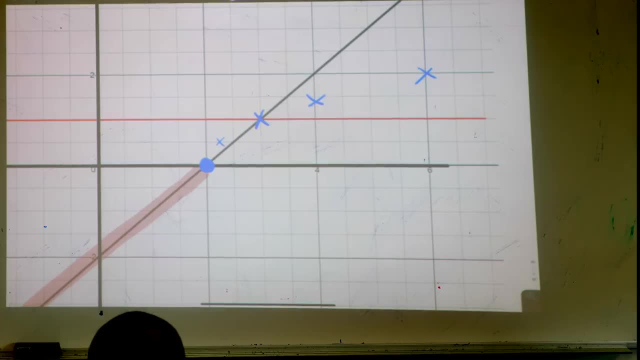 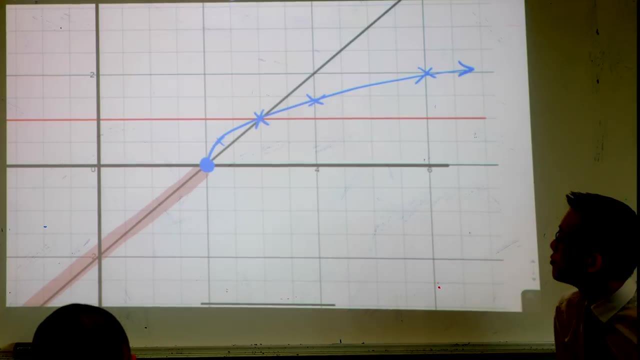 You could put in a few more points if you were confident, But I'm pretty sure this is starting to look like this kind of shape, Like: so What do you think of that? Are you happy with that? Like, I've joined up the dots. 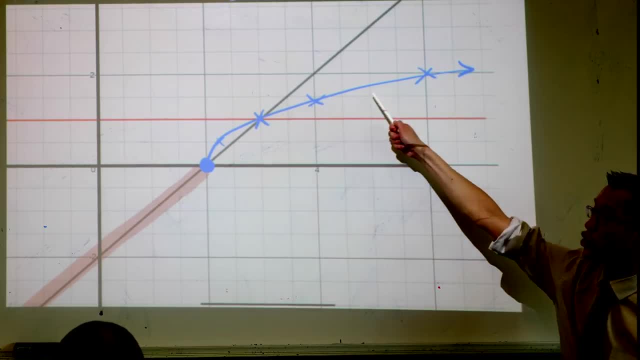 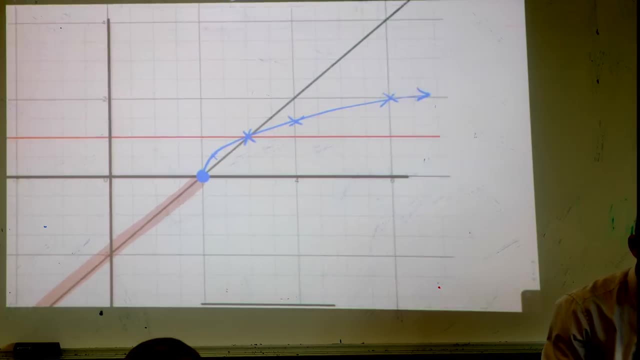 You can see they're steeper earlier on and then it kind of like shallows out over here Now. hopefully, when you look at this, this shouldn't be too much of a surprise for you, Right? Because we've actually dealt with functions like this before. 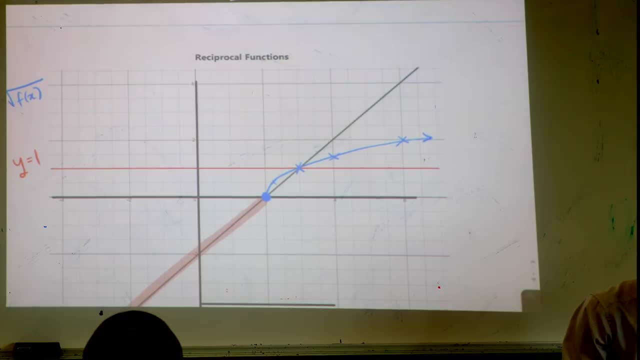 Sorry, this is not reciprocal functions. I was just cheating and using the same page, So I'm just going to get rid of that. There we go, This graph here. Can someone tell me what the equation of this graph is? y equals.